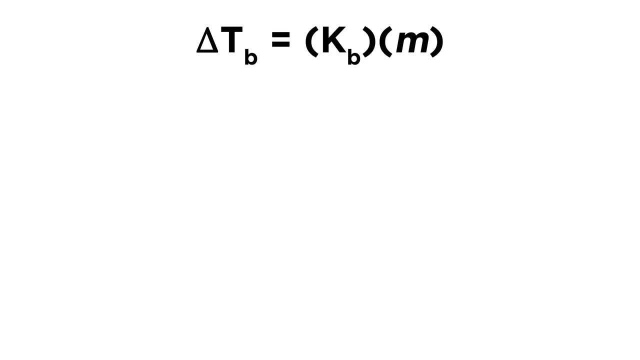 delta Tb We're going to find the change in the boiling point from the boiling point of pure benzene And that is going to be equal to the Kb for benzene times the molality. And so we're given this information, We just plug it in: Delta Tb is equal to the Kb for benzene times the molality. 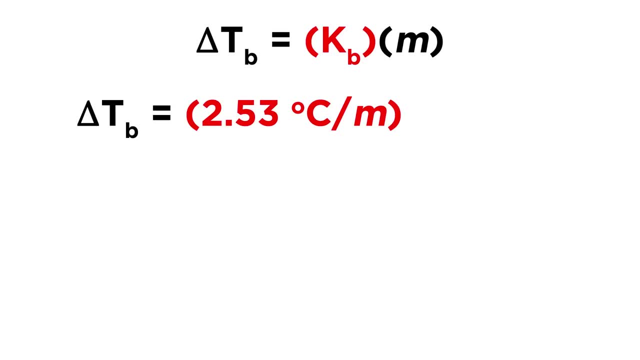 Delta Tb is going to be equal to Kb for benzene, which is 2.53 degrees Celsius per molal, And we were told that the molality of the solution is 0.33 molal. So that is what is given. We can then calculate delta Tb. That is going to be equal to 0.83 degrees Celsius. 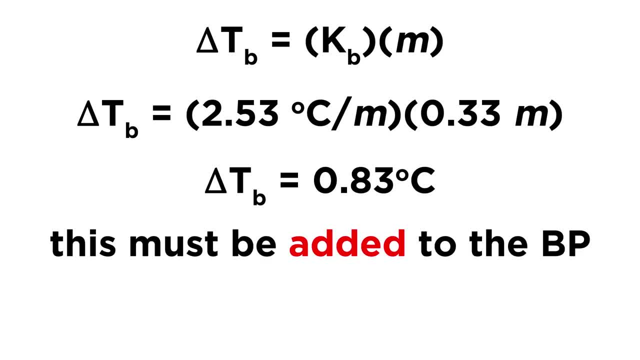 And what we must be aware of is that delta Tb, that change in boiling point, must always be added to the boiling point, And so we're going to find the change in the boiling point And that is going to be equal to the boiling point of pure solvent, Because the presence of 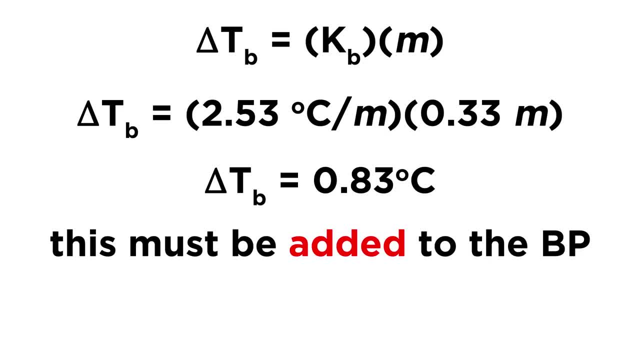 solute in a solution will always cause a boiling point elevation. It will always cause the boiling point to increase. And so 80.1 degrees Celsius, which is the boiling point of pure benzene plus 0.83 degrees Celsius, or the boiling point elevation, or the change in boiling point. 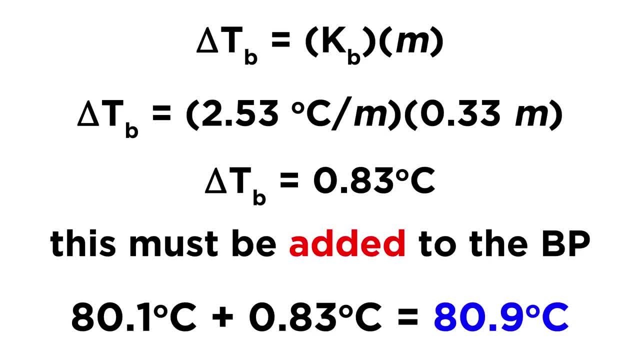 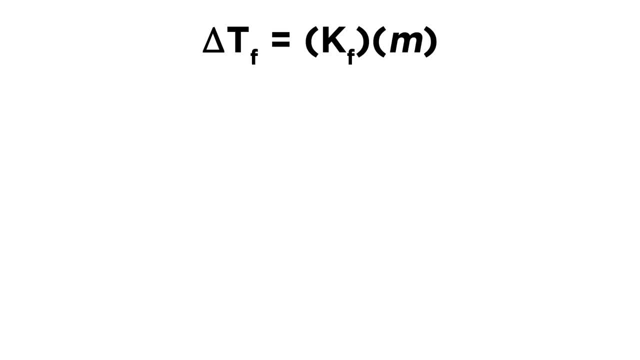 that gives us 80.9 degrees Celsius. So that will be the new boiling point for this solution. Now let's look at the other question. For the other question, we're trying to find a freezing point, So let's use delta. Tf equals Kf times molality, So it's pretty much the same. We're 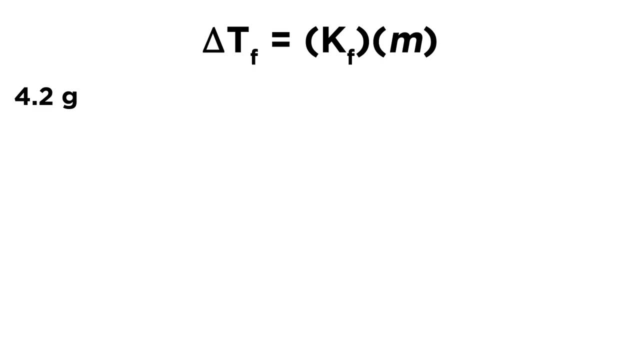 just finding the change in freezing point now, And so we were given 4.2 grams of NaCl, And so what we need, though, is molality, And molality involves moles, not grams for the solute, So 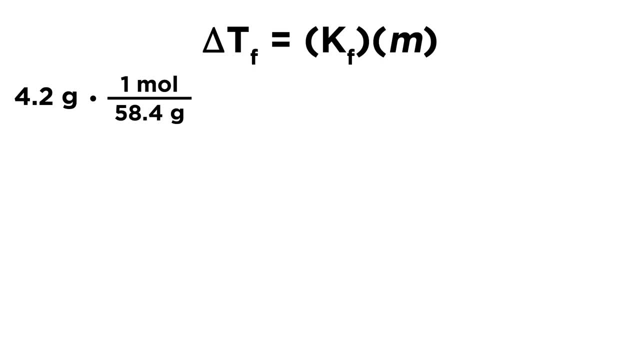 let's multiply that by 1 mole over 58.1 degrees Celsius And we're going to find the change in 8.4 grams. That's the molar mass of NaCl, And so from that we realize that we have 0.072 moles. 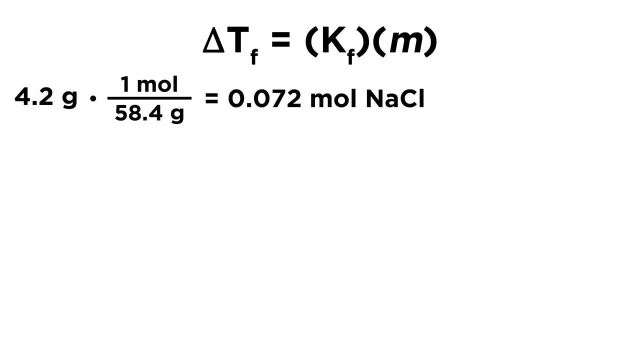 of NaCl. But here is a very critical step. We have to realize that when we put NaCl into aqueous solution it is going to dissociate. It is going to dissociate into sodium ions and chloride ions. And so if we have 0.072 moles of NaCl, 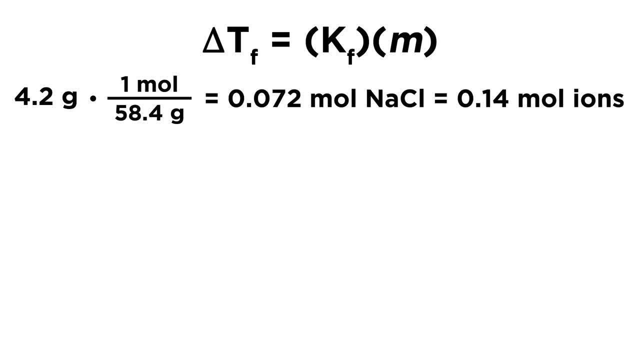 once those ions dissociate from one another, we are going to have precisely twice as many moles of ions in general, And we need to know the moles of particles, of solute particles that are in solution, because that is going to give us our molality. So we need to know. 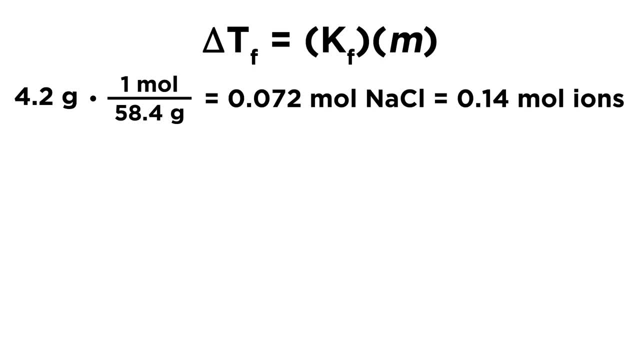 that we have to double this value in order to get the moles of ions. Now that we have the moles of ions that are in solution, we're ready to calculate molality. And so, remember, molality is moles solute per kilogram of solvent, And we have 0.14 moles of solute And we had 125 milliliters of. 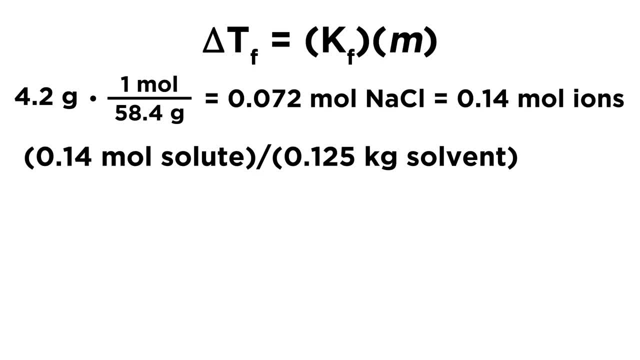 water. That was our solvent, And so 125 milliliters is the same as 125 grams, which is the same as 0.125 kilograms of solvent. So we needed to convert our volume of solvent into a mass in kilograms. That's how we get molality And we find out that the solution is 1.4.. 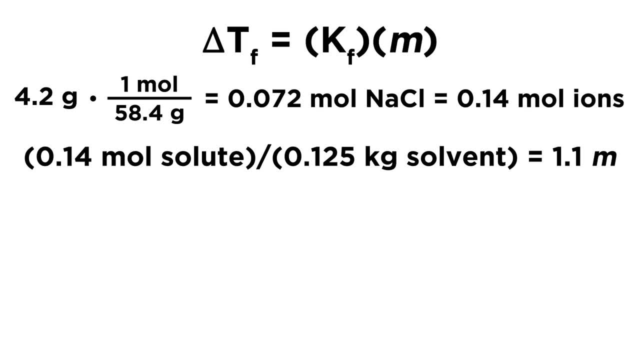 Molal. So now we're ready to plug things in. So delta Tf is going to be equal to 1.86 degrees Celsius per molal. That is the Kf value for water, And then we have just calculated our molality as. 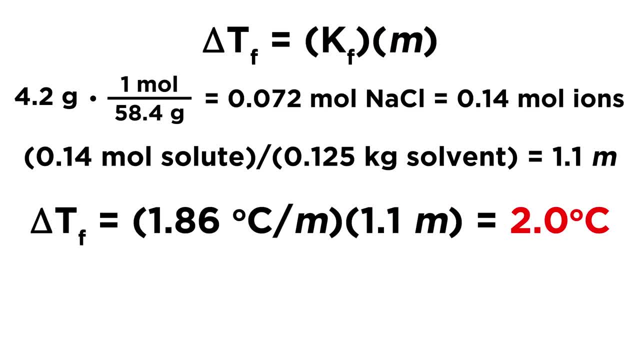 being 1.1 molal, And so if we do the arithmetic we get 2.0 degrees Celsius. That is the change in freezing point for the solution from the freezing point of pure water. Now we have to realize that this must be subtracted from the freezing point of pure water. 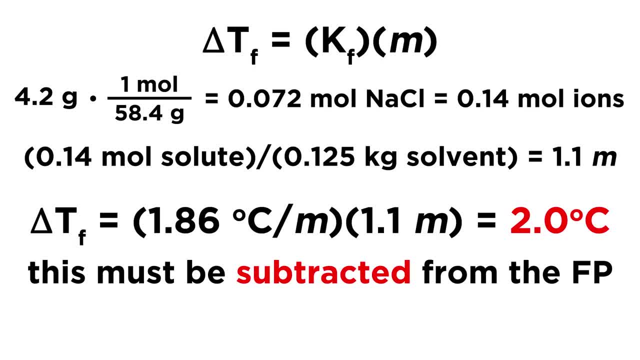 because the presence of solute in solution will always cause freezing point depression. It will cause the freezing point to lower from the freezing point of the pure solvent, And so if we subtract that- we know that water typically freezes at 0 degrees Celsius- We can then subtract 2.0 degrees.